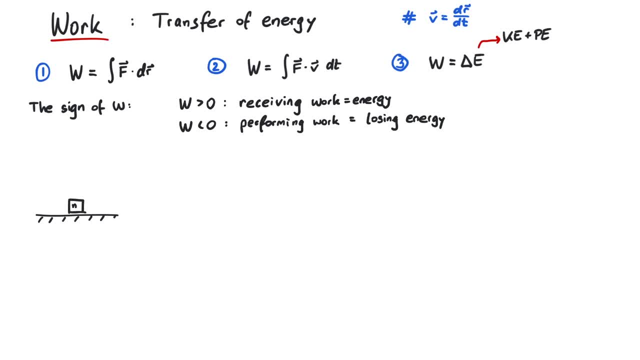 Imagine an object of mass m sitting on the ground. In order to raise it to a height h above ground, we have to apply the force mg in positive z-direction And the path that the object is traveling is purely the z-direction, within the boundaries of zero and h. 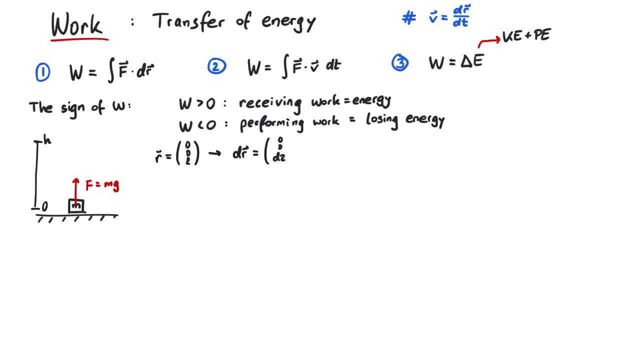 This means our differential path is just And the dot product simplifies to the integral between zero and h over mg times dz, This yields mgh, which has units of energy. The work we just calculated is positive. therefore it is absorbed by the object as potential energy. 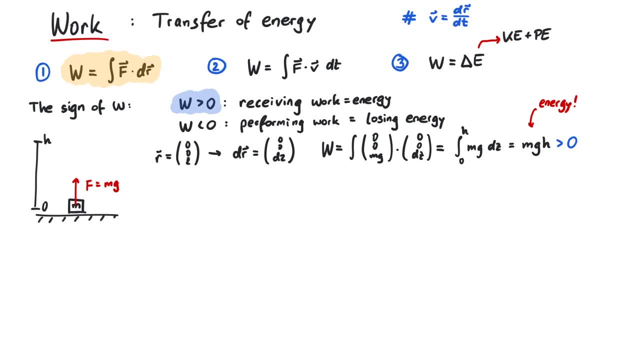 Since forces always come in pairs, thanks to Newton's third law, the same process that led to an increase of energy must lead to a decrease of energy somewhere else. Now consider the hand that is raising the object. If you pick it up, you experience the force. 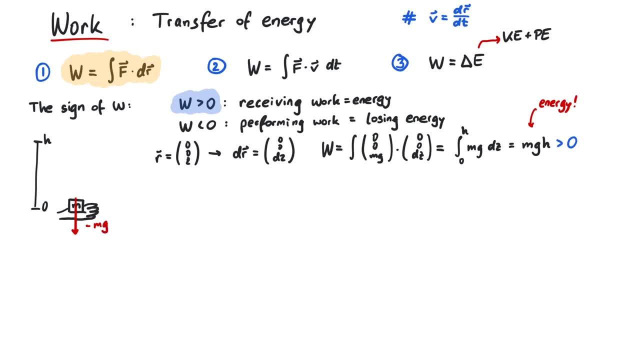 minus mg pressing down onto your hand. This is just the weight of the object you feel on your hand. Since the force now has opposite sign, we get the same numeric result but with a minus sign. So the action of moving your hand to the height h corresponds to giving energy away. In other words, 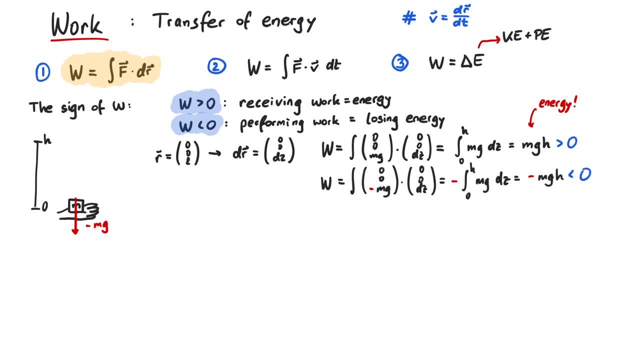 you transferred the chemical energy stored in your muscles to potential energy of the object. Note that if the force vector and dr are perpendicular to each other, then no work is being performed. If you carry something from point A to point B, where A and B are on the same altitude, 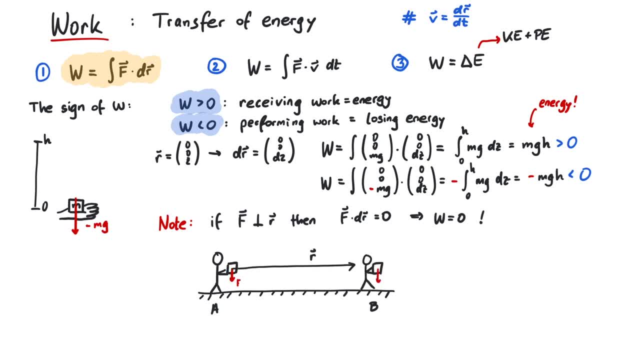 then you might be exhausted, but in the physical sense you haven't been doing any work. So now that we know about work, we can also talk about power. Power is a measure for how much work has been performed in a certain time. 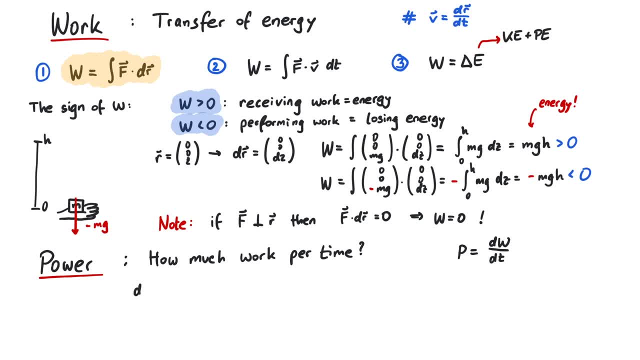 Let's take our previous example. Imagine we raise the object in 10 seconds, Then the power of this action is mgh divided by 10.. Now imagine we do the same process, but very slowly, Say we need 10 minutes for this, Then the corresponding power is mgh divided by 600.. As you can. 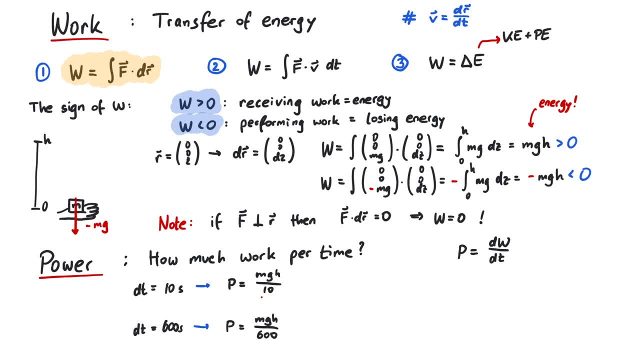 see, if you do the same work in less time, then your required power is larger, And that's pretty much it for this time. Thanks for watching.